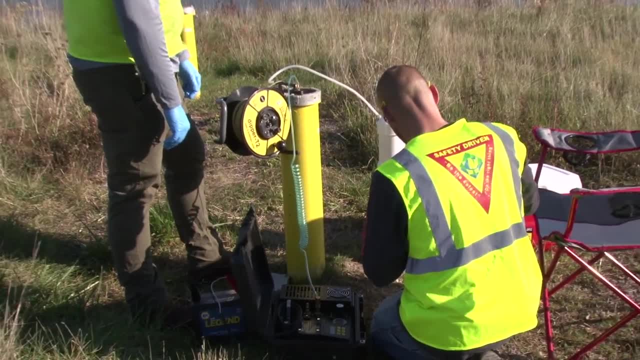 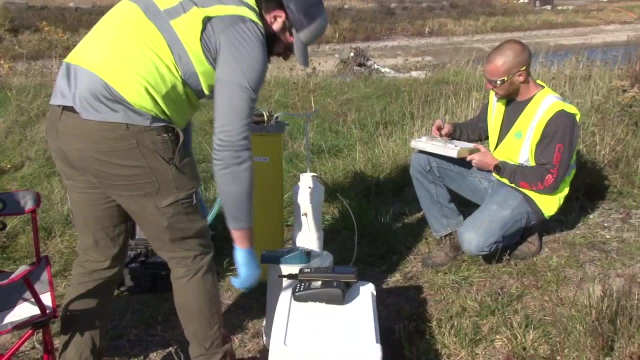 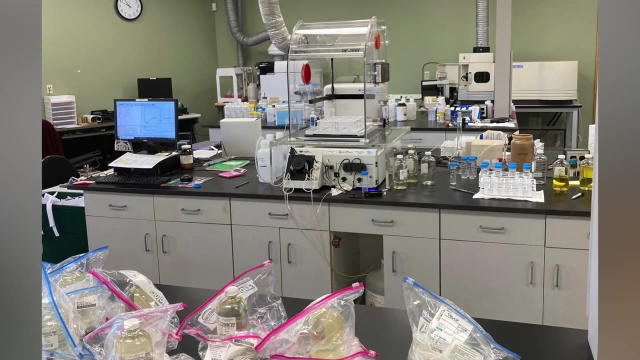 analytical plan. These plans, which were developed with the guidance and approval of the New York State Department of Environmental Conservation, provide the methods and procedures that ensure the proper collection and handling of samples, the chemical analysis of samples, reporting of laboratory data and the 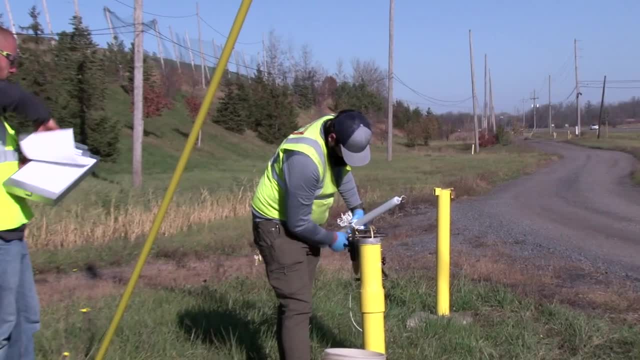 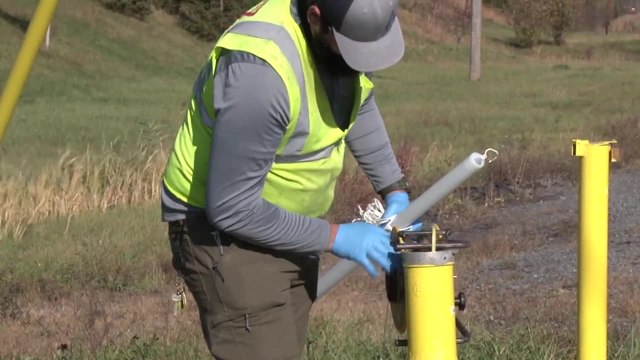 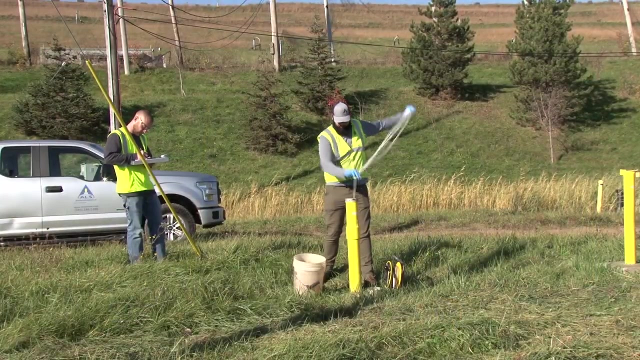 evaluation of the laboratory data. The Tablet Monitoring Program helped to assess groundwater quality at the facility once analyzed at an Indian Ocean doener facility. Our activities were 조 and. the monitoring of groundwater quality at the facility is accomplished with the analysis of groundwater sampled at 33 shallow wells and 27 deep wells that extend into the bedrock beneath the site and around the perimeter of Seneca Meadows. 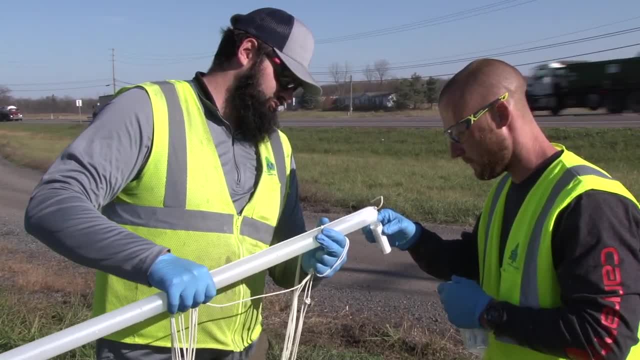 The all of the wells in place are approved and permitted by the DEC. The well depths range from about 15.5 diM diff out of 800.com To survive사 to survive lighter waters without stopping, as hopefully. kurt certainly thought something else for the Jana and Homerio力 geo ducks, but that full west is that day. off the depots. 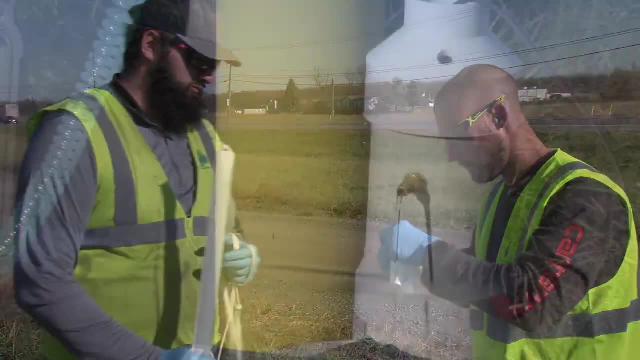 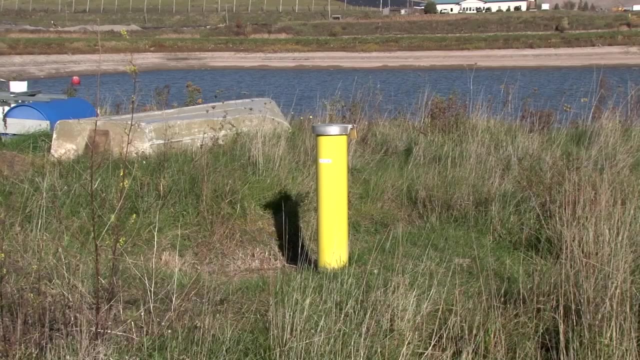 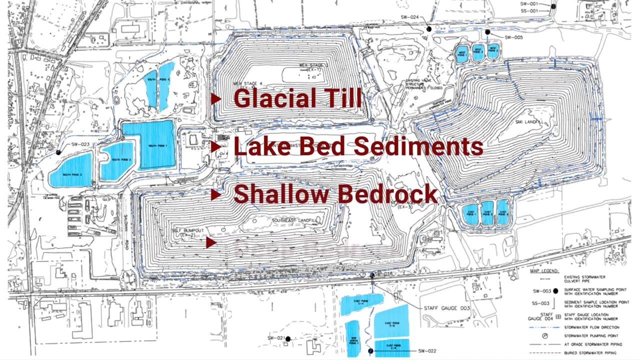 feet to more than 120 feet. The wells are two inches in diameter and are constructed of PVC. Each well allows for the collection of samples from a given geological zone, For example glacial till lake bed sediments, shallow bedrock and deep bedrock. These analysis confirm that the 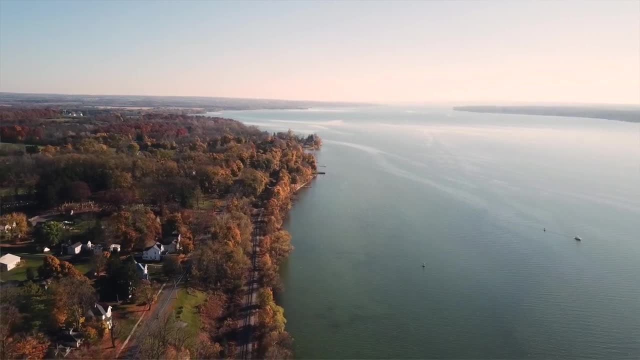 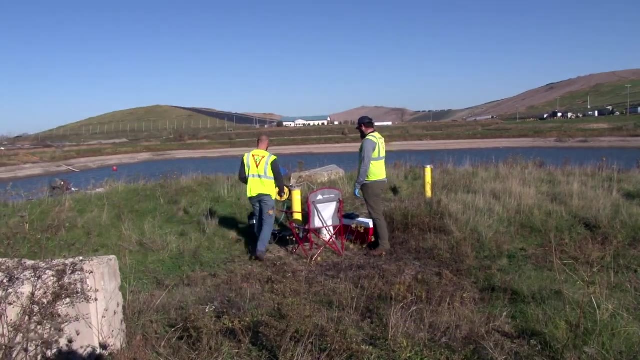 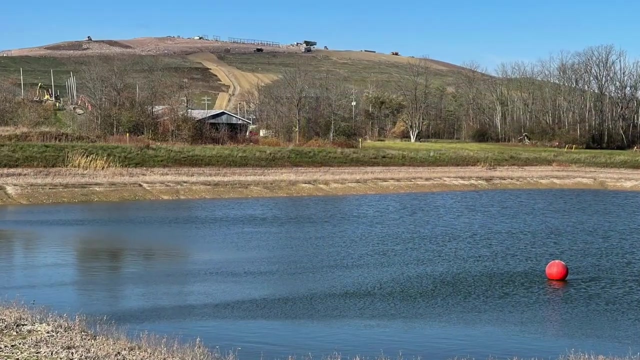 active landfill is not negatively impacting the groundwater quality in the surrounding area. Seneca Meadows monitors stormwater and natural surface water quality in accordance with New York State's Speedy's multi-sector general permit for stormwater discharges associated with industrial activity and its part 360 operating permit through the DEC: Our operating permit. 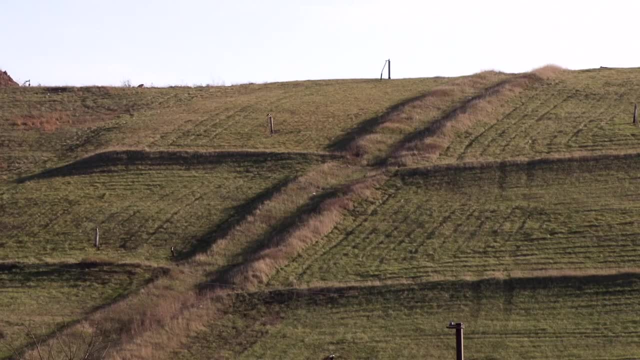 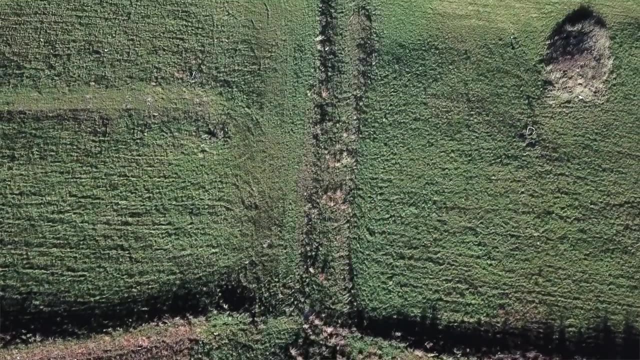 requires the collection, sampling and discharge of runoff within the existing landfill footprint, as well as what leaves the landfill footprint. The multi-sector general permit requires the monitoring of runoff from portions of the site that are associated with industrial activities. The monitoring of the 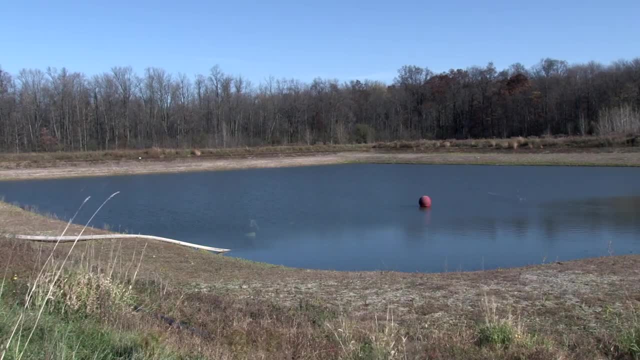 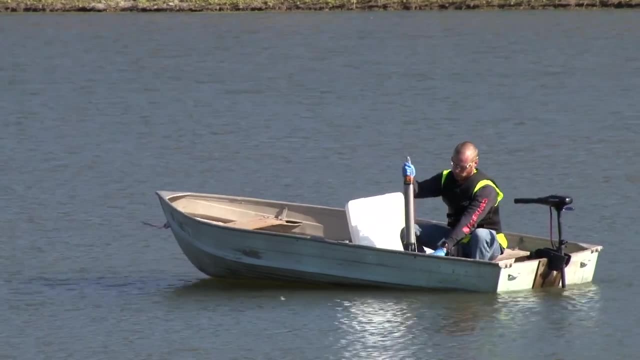 stormwater retention pond systems is accomplished with the analysis of the retained water prior to discharge. Discharges from these retention ponds occur after the stormwater runoff has been stored for at least two weeks, has been sampled and analyzed has had results compared to the 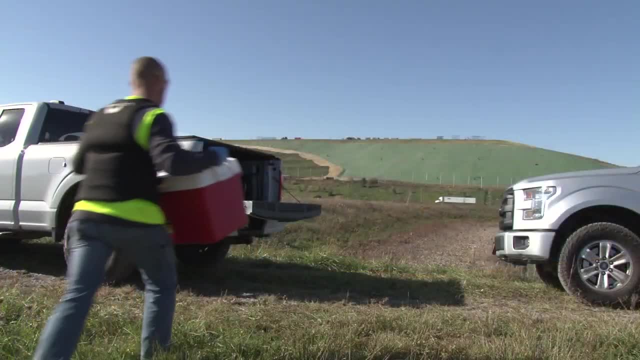